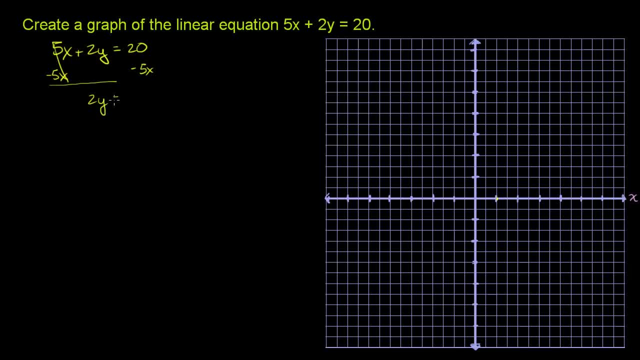 The left-hand side. these guys cancel out. So we get: 2y is equal to the right-hand side. You have 20 minus 5x, And then you could divide both sides of this equation by 2.. So you divide both sides by 2.. 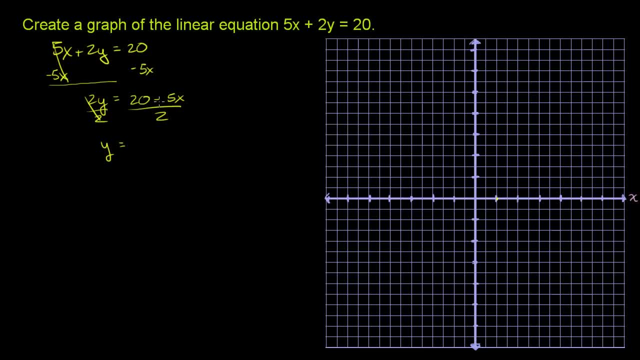 The left-hand side we just have a y And then the right-hand side. we could leave it that way. That actually would be a pretty straightforward way to leave it. But we could call this: 20 divided by 2 is 10 minus 5x over 2, or minus 5 halves times x. 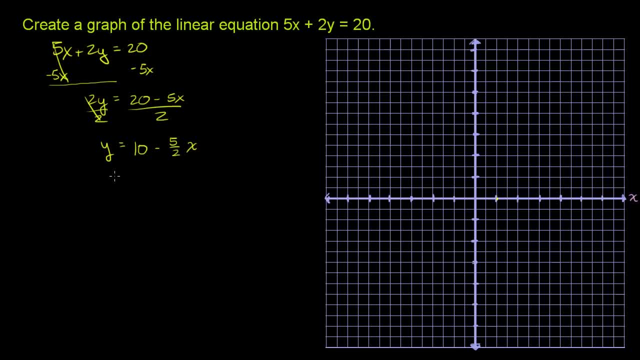 And so now, using this, let's just come up with a bunch of x values and see what the corresponding y values are, and then just plot them. So let me do this in a new color, So let me a slightly different shade of yellow. 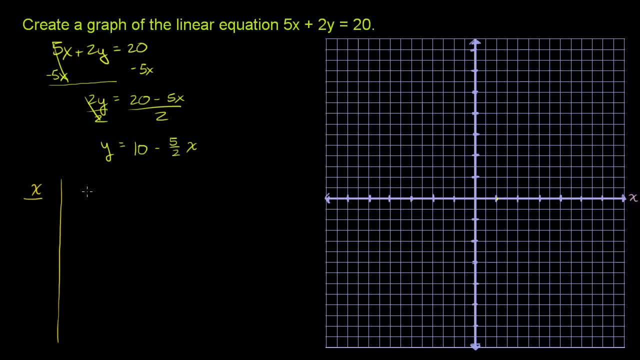 So we have x values, And then let's think about what the corresponding y value is going to be. So I'll start. well, I could start anywhere. I'll start at x is equal to 0, just because that tends to keep things pretty simple. 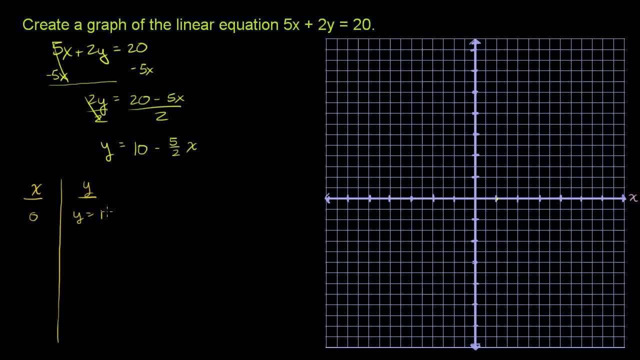 If x is 0, then y is equal to 10 minus 5 halves times 0,, which is equal to 5 halves times 0, is just 0. So it's just 10 minus 0, or 10.. 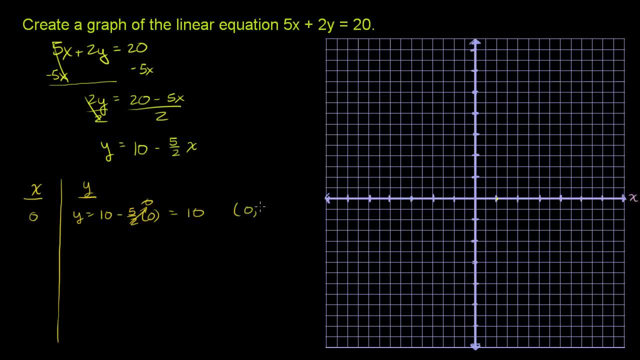 So that gives us the coordinate, the point 0, comma 10.. When x is 0,, y is 10. So 0,, so x is 0, so it's going to be right here in the middle of the x-axis. 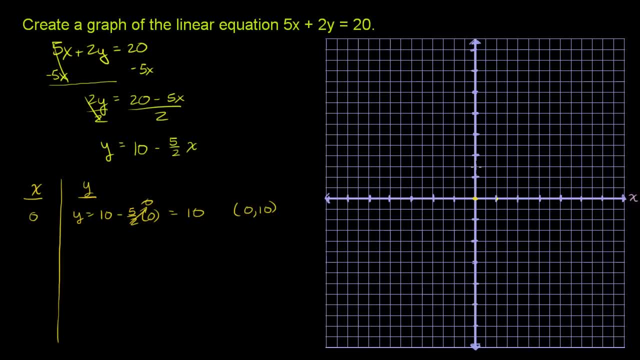 And you go up 10 for the y-coordinate 1,, 2,, 3,, 4,, 5,, 6,, 7,, 8,, 9,, 10.. So it's right over here. So that's the point 0, comma 10.. 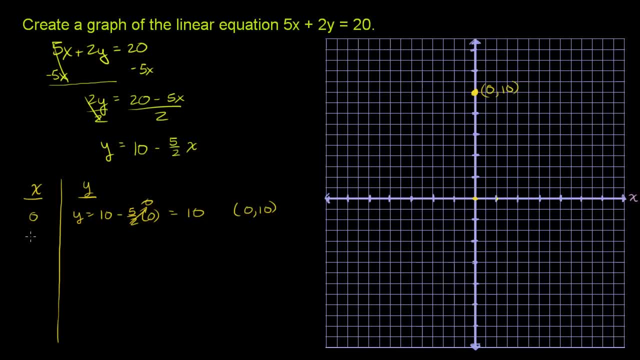 Let's do another point. Let's say that x is 2.. I'm going to pick multiples of 2 here, just so that I get a nice clean answer here. So when x is 2, then y is equal to 10 minus 5 halves times 0.. 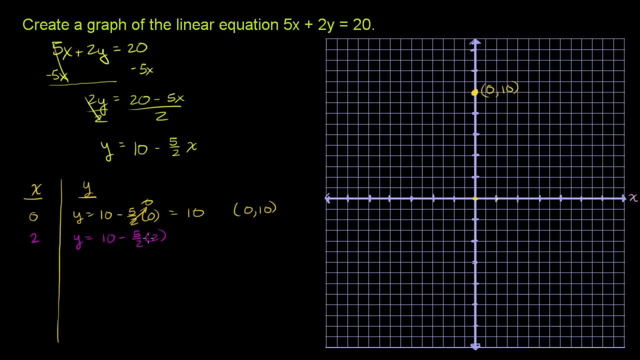 OK, 2 halves times 2.. And the 2 in the denominator cancels out with this 2 in the numerator. So it simplifies to 10 minus 5, or just 5.. So that tells us the point: x equals 2, y is equal to 5,. 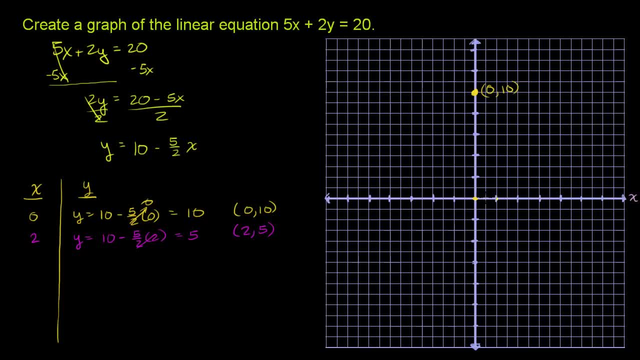 is on the line. So 2, x is equal to 1,, 2, right over here- And then y is equal to 5.. You go up 5.. 1,, 2,, 3,, 4,, 5, just like that. 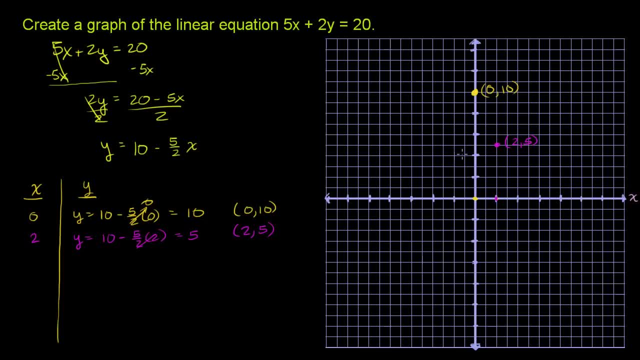 So that's the point 2, 5.. And when you're drawing a line you actually just need 2 points. If we have a ruler or any kind of straight edge, we can just connect these 2 points And if we do it neatly, every point on that line. 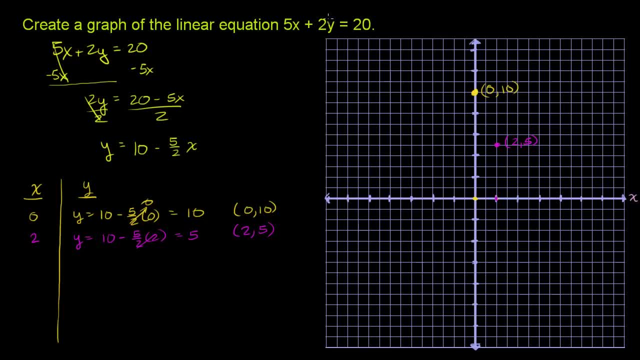 should satisfy this relationship right here, Just so we get practice. I'll do more points, So let me do. let's say: when x is equal to 4, then y is equal to 10 minus 5 halves times 4.. This is equal to 5 halves times 4.. 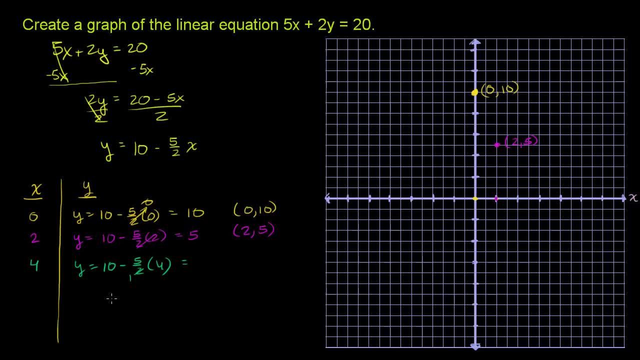 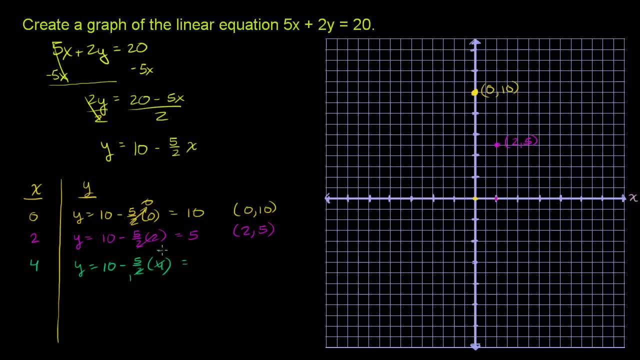 So that's the point. Divide the denominator by 2, you get 1.. Divide the numerator by 2, you get 2.. Or 4 over 2 is the same thing as 2.. So it becomes: 2 times 5 is 10.. 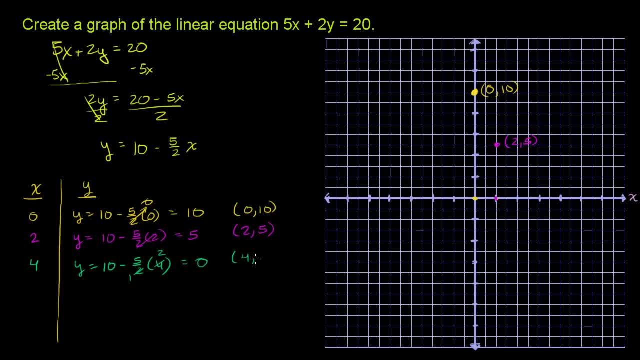 10 minus 10 is 0. So the point 4, comma 0 is on our line. So x is 1,, 2,, 3,, 4. And then y is 0. So we don't move up at all. 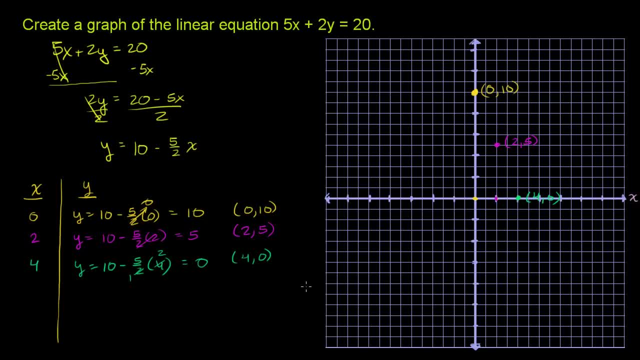 So we have 4, 4 comma 0. And I could keep going. I could try other points. You could do them if you like, But this is plenty. Just 2 of these. 2 of these would have been enough to draw the line. 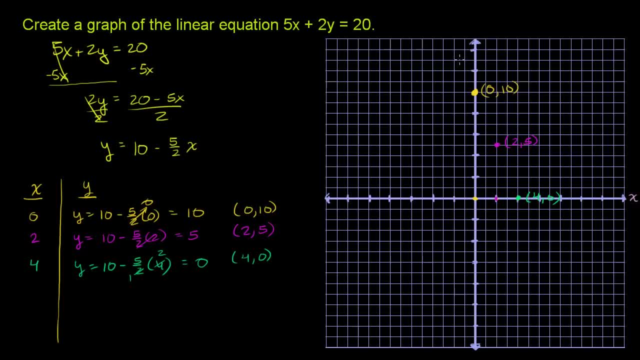 So let me just draw it. So I'll do it in white. So the line will look something like this, The line will look something like that, And I could keep going in both directions. So there you have it. That is the graph of our linear equation. 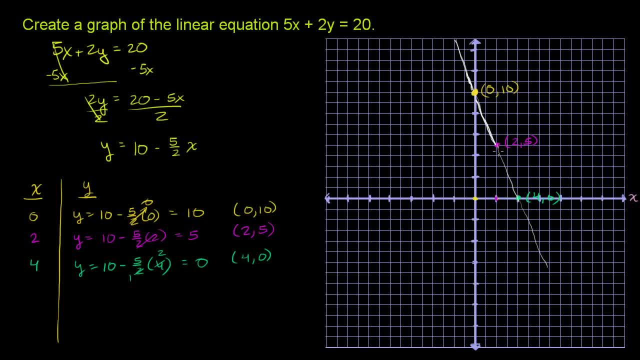 Let me make my line a little bit bolder, just in case you found that first line hard to read. So let me make it a little bit bolder And I think you get the general idea.